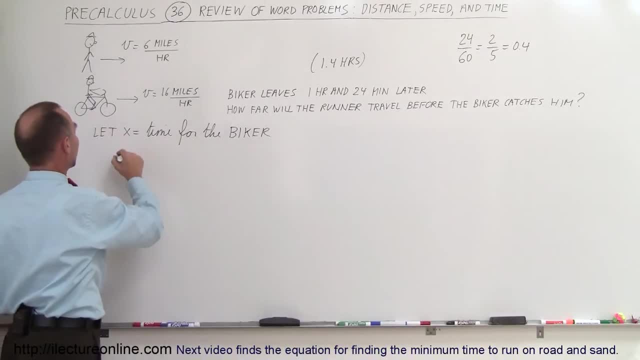 on the road will be X, the amount of time for the bike plus 1.4 hours. So X plus 1.4 equals the time for the runner. Ok now, the principle here is that when the biker finally catches the 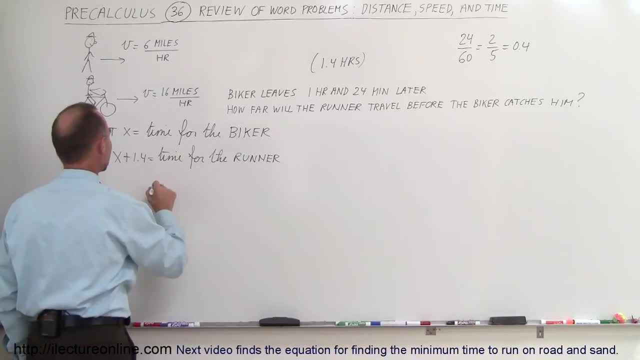 runner, they will have covered the same amount of distance. So the distance covered by the runner must equal to the distance covered by the biker, And that's how we're going to work out this problem. And then, of course, you have to realize that distance equals velocity times time. 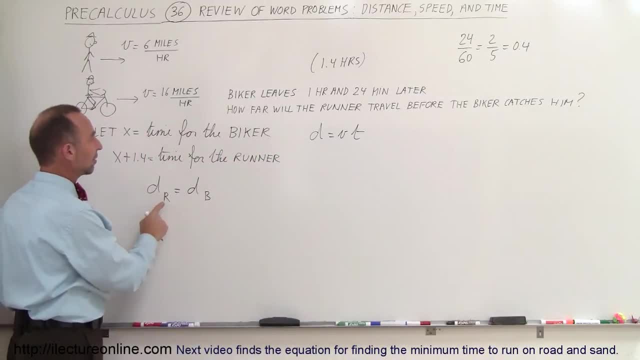 So in this case the speed of the runner times the time of the runner is equal to the speed of the biker times the time of the biker. So the speed of the runner is six miles per hour and the time for the runner would be X. That equals the speed. 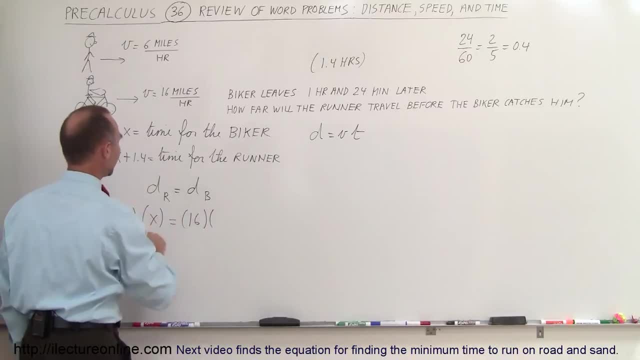 of the bike, which is 16 times the time for the bike, which would be: oh no, no, I got this wrong here. runner spends more time, that's the biker. the runner spends more time on the road, so I want six times X plus 1.4.. 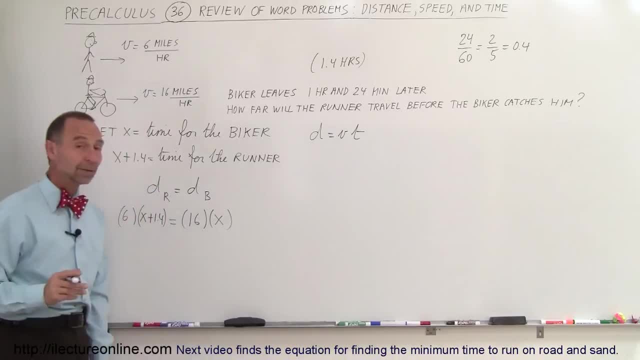 And 16 times X. that's the most appropriate one, right, because the runner spends more time on the road than the biker. Alright, now we have to solve this equation for X, and so let's go ahead and get rid of parentheses. 6X plus 6 times that would be 8.4- equals 16X. 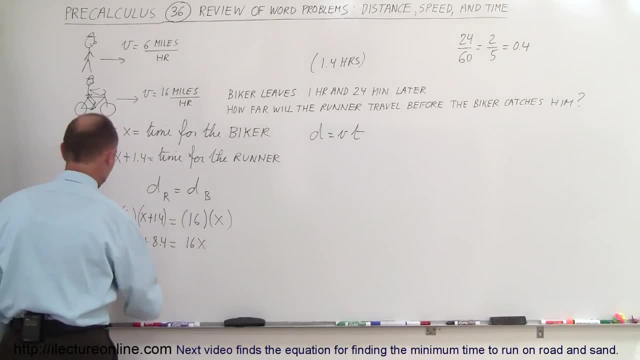 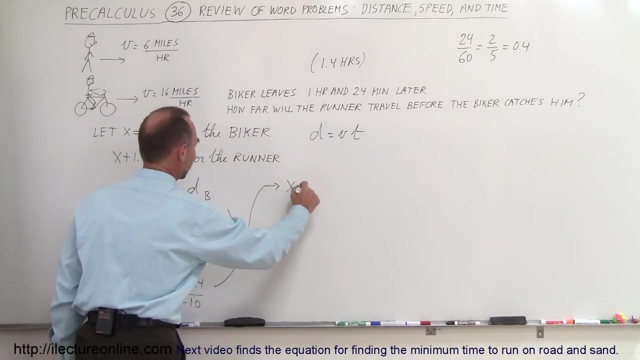 Moving all the X's to one side, all the numbers to the other. So we have 6X minus 16X equals minus 8.4.. So minus 10X equals minus 8.4, dividing both sides by the coefficient minus 10, that gives us X is. 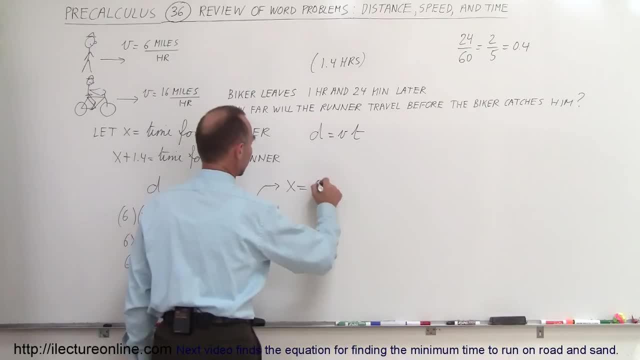 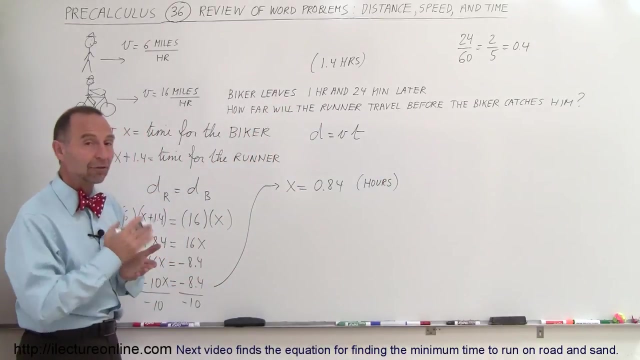 equal to 0.84.. Okay, 0.84X is the time for the biker, so that would be 0.84 hours on the road for the biker. So from that we can figure out how far the biker will have traveled. 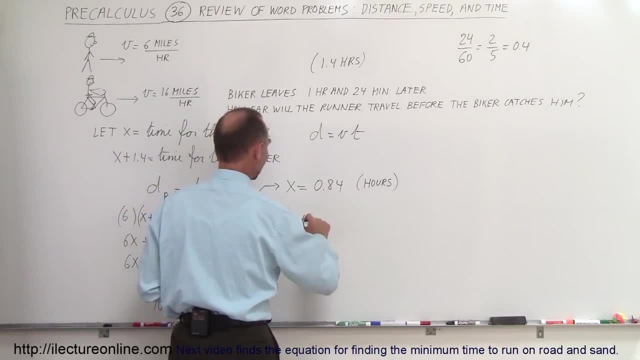 before catching the runner. And so, since you know that distance equals velocity, times time, and for the biker the velocity is 16 miles per hour times the time, which is 0.84.. And let me get a calculator out for that.